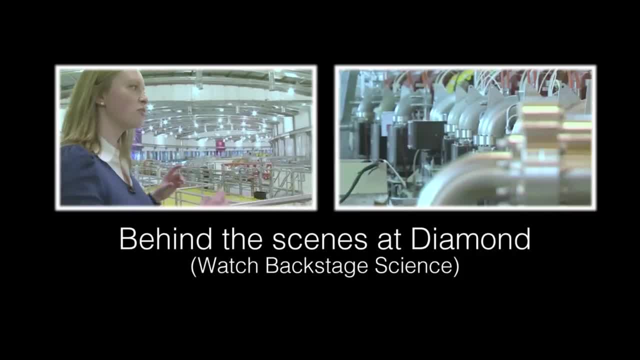 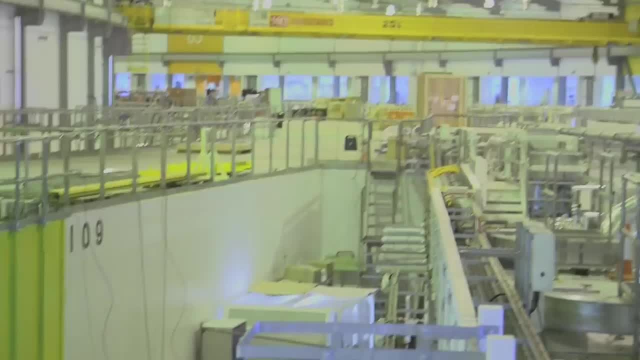 We walk around as there's a sort of hissing noise, and the hissing noise comes from nitrogen gas. Now, because of this very bright light that we have, it's very, very focused, but it can get quite hot. So we are standing right above what is called beamline I09.. What's a beamline? Well, 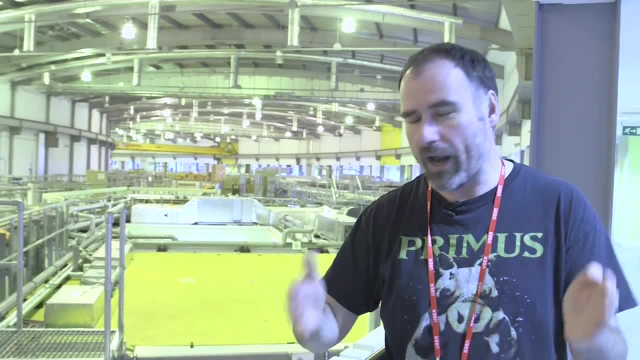 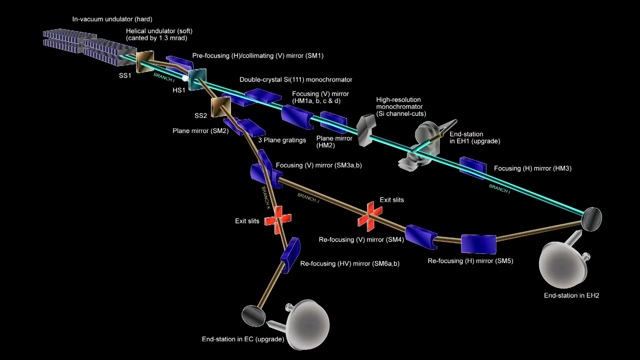 you have the electrons circulating around, How do you get the light out? Well, what happens is you have tubes, funnels, through which the light travels, And those are, as you can see, going off into the distance. you might be able to see this in 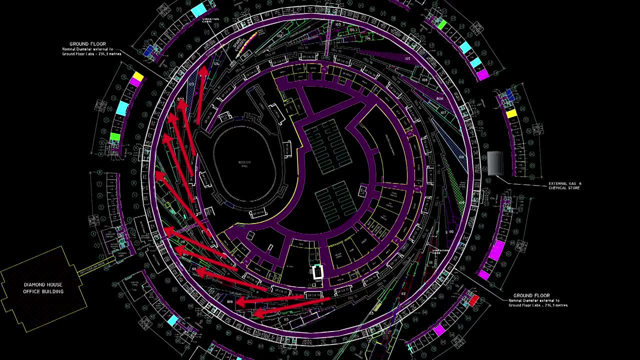 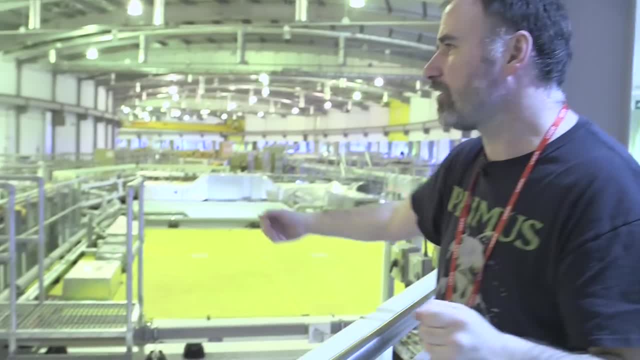 terms of just coming off tangentially to the ring. We're on the surfaces and interfaces line just here, just down here, And we will be collecting that light coming from those electrons and shining it onto our sample down in this experimental hutch down here. 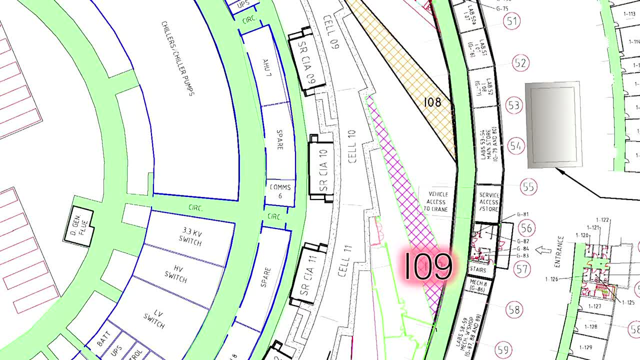 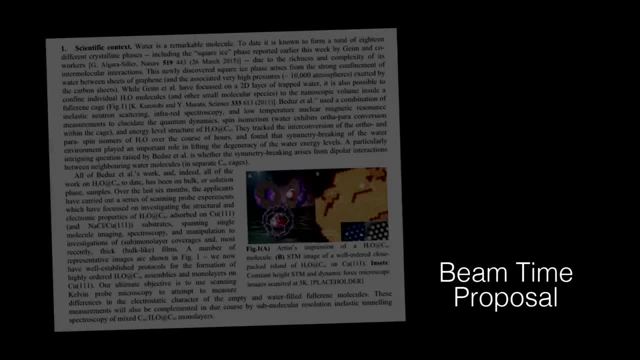 So to get beam time, you have to like anything in science, you have to write a grant proposal, You have to get the time, You have to get the funding For the work. And we wrote that proposal quite some time ago, almost a year ago now. 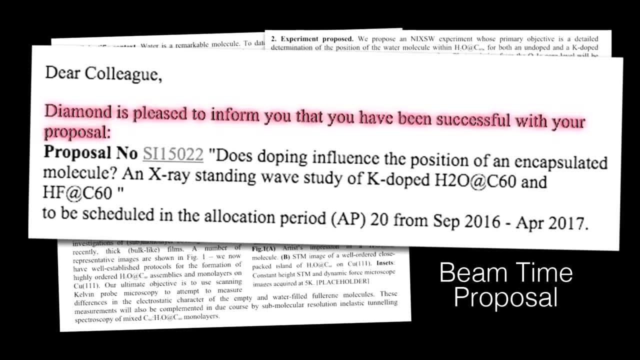 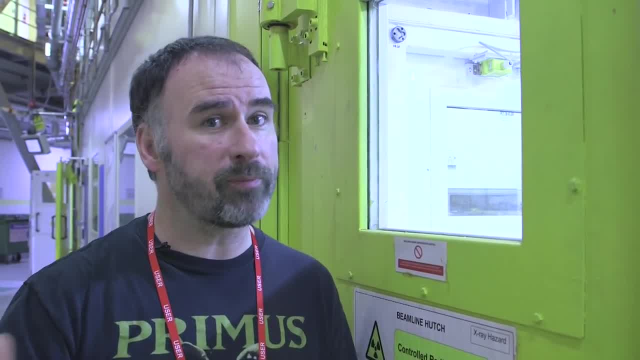 So we were hugely excited when we got the time and now we're hugely excited to be here to actually be able to exploit this synchrotron radiation. So what we're looking at here is, obviously we need to have optics to get this light down. but this is optics, These are X-ray optics. 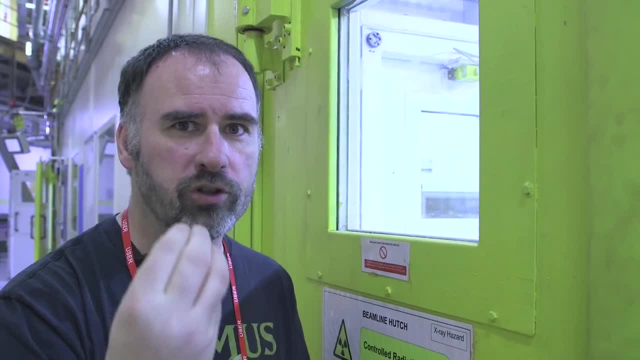 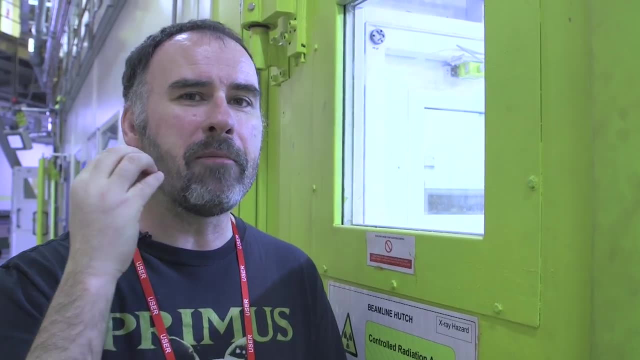 and we need to be able to get those X-rays onto our sample to focus them down. The synchrotron is about 10 billion times brighter than the sun, So this is an immense engineering challenge, with very, very clever people doing this work. 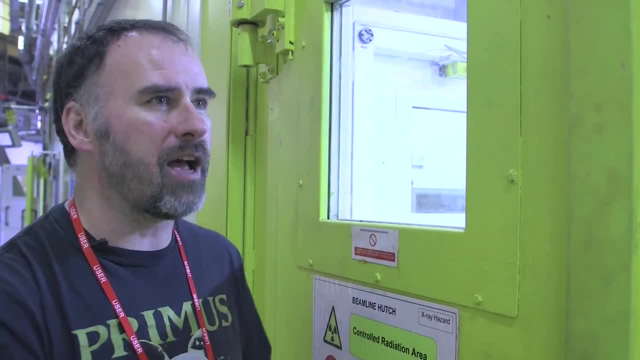 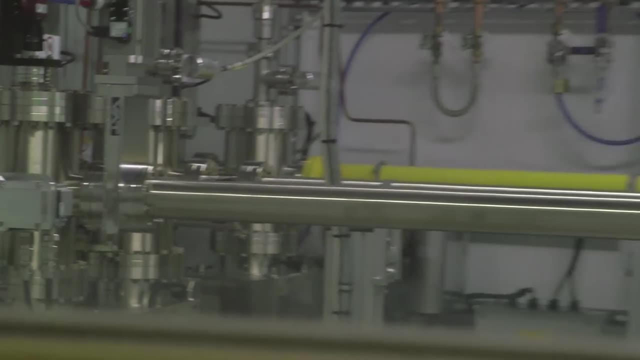 to ensure that we can get those very bright X-rays and get them onto our sample. So the tube you can see coming down here is actually the tube that is carrying the beam to our chamber And it's all ultra high vacuum, So it's a pressure comparable to that you get on. 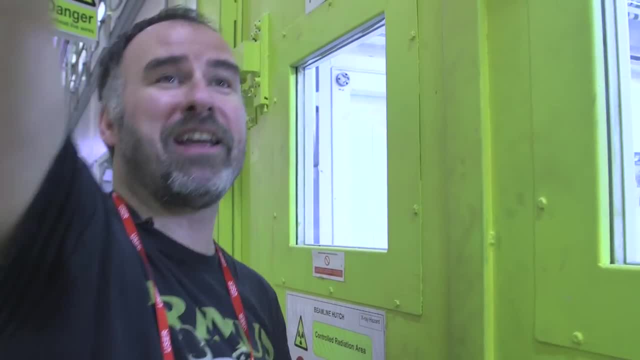 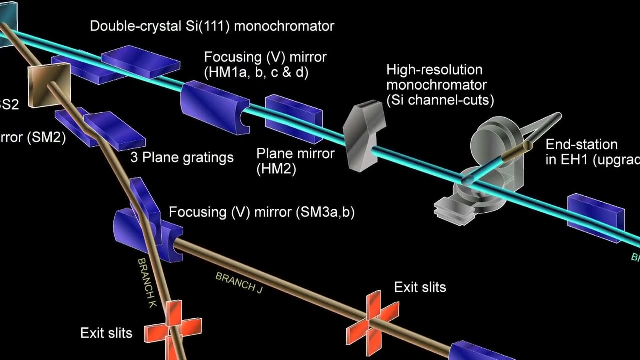 the surface of the moon. The electrons are not in that tube. The electrons are busily circulating away over there. What is coming down this tube is the light generated by those electrons And that's going to come into our Earth. similarly, ultra high vacuum chamber, We're going to have those X-rays and they're going to impinge on our 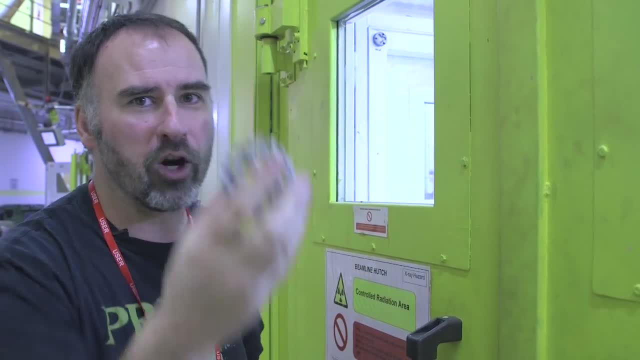 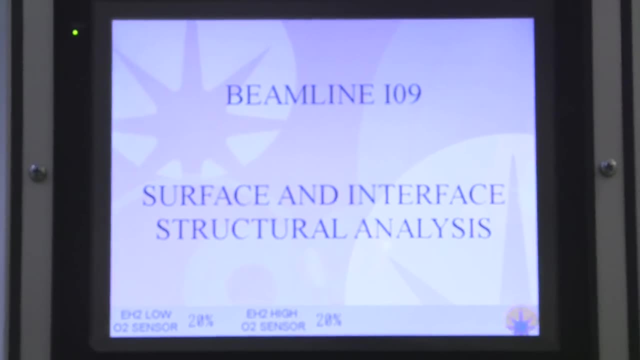 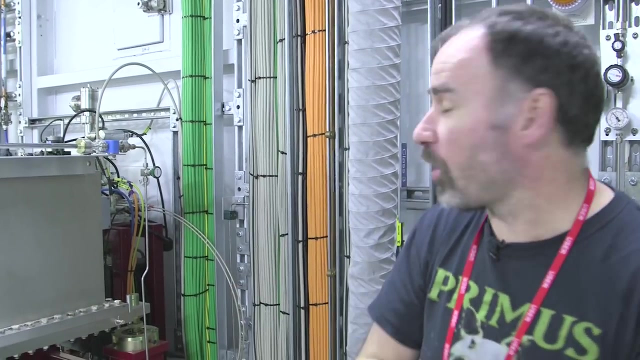 sample, And then we're going to find out wonderful things about our particular molecule. We're in the experimental hut. This is where we actually do the experiments, And the light actually comes in through this tube here, And then we're going to chase that through. We've 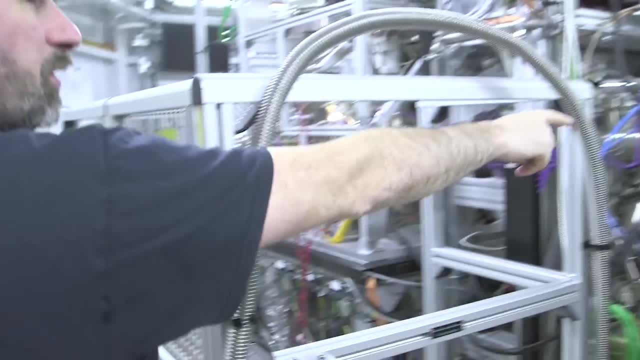 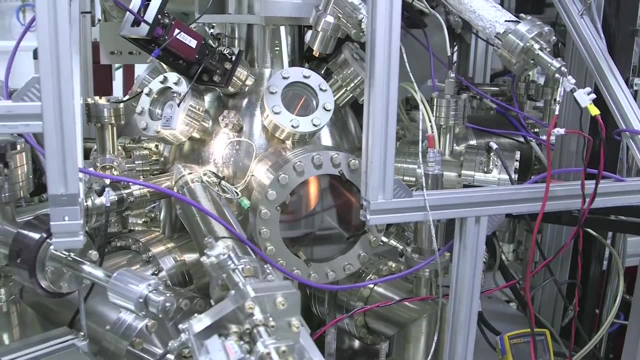 got some mirrors et cetera, some more optics, some types of diagnosis, And then we're coming all along, all along into our experimental chamber here. It's an ultra high vacuum chamber, stainless steel. Pressure in here very, very low again. 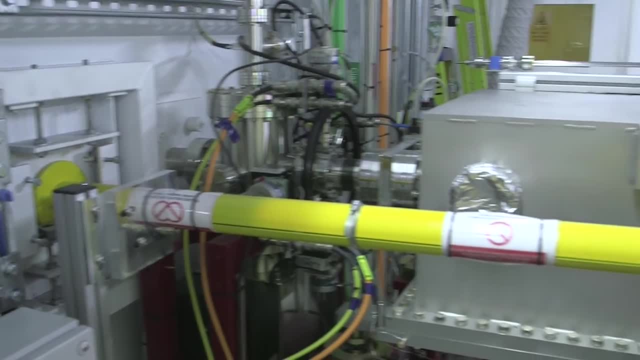 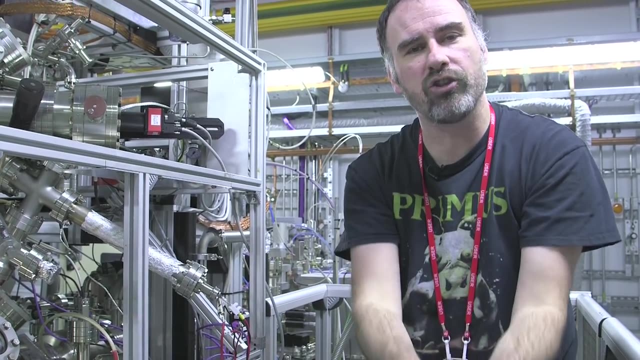 comparable to the surface of the moon And our sample sits in there. So the beam is coming into our chamber And the beam is going to hit our sample and it's going to eject electrons out And we want to measure the energies at which those electrons come out. It's actually something called. 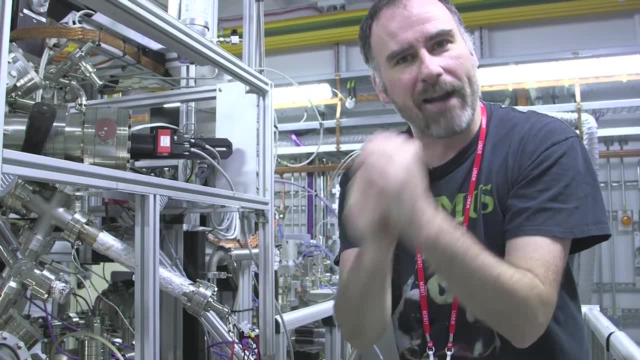 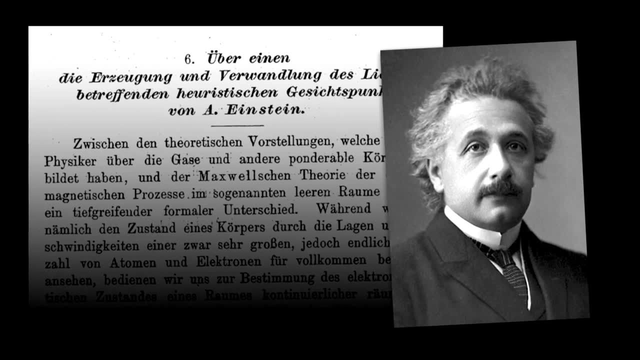 the photoelectric effect, which is the relativity, that Einstein won his Nobel Prize. It was actually for the photoelectric effect, something called photoemission. That's what we're doing here, One part, it's just one part of what we're doing here. Photons in, electrons out, And every material. 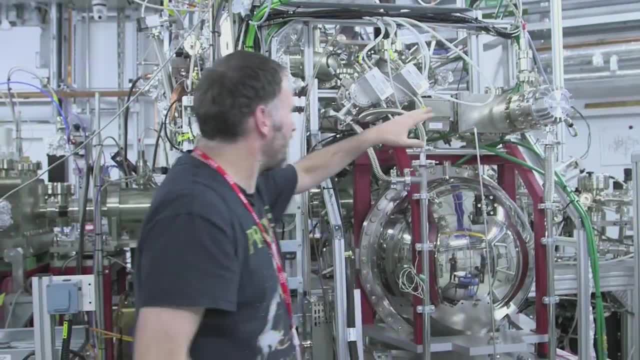 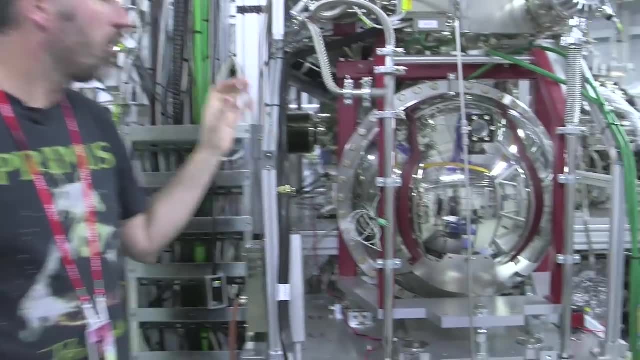 has its own signature in terms of its photoemission spectrum. So this is our electron energy analyzer, this wonderful hemispherical analyzer, And it's literally called a hemispherical analyzer. And the way we measured the energies of the electrons is that we have a 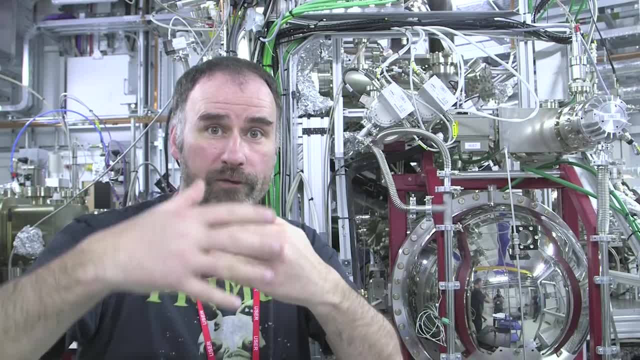 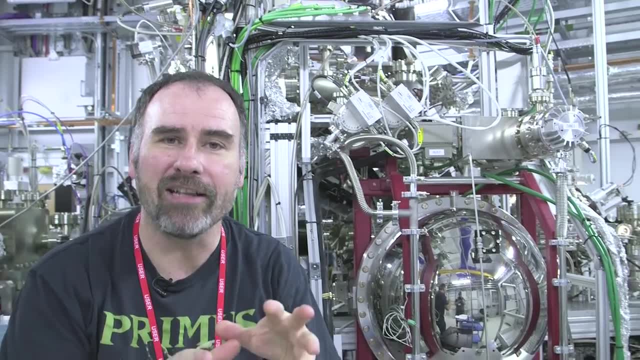 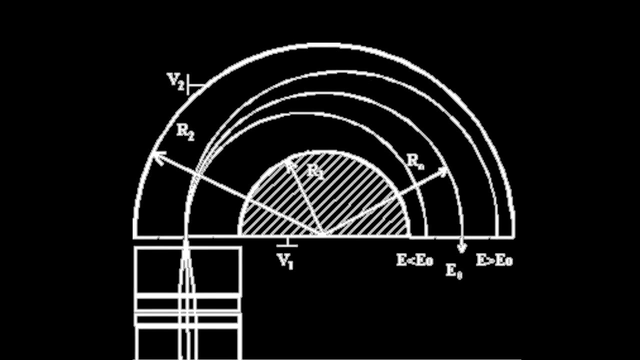 couple of spheres in here and we put a voltage on those spheres And then what we do is we play off the centripetal force on the electrons against that voltage. So we play off the centripetal force against the electrostatic force And only those electrons that have got the right kinetic energy, the right speed. 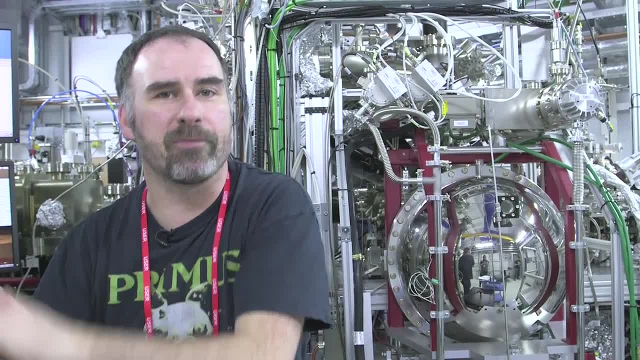 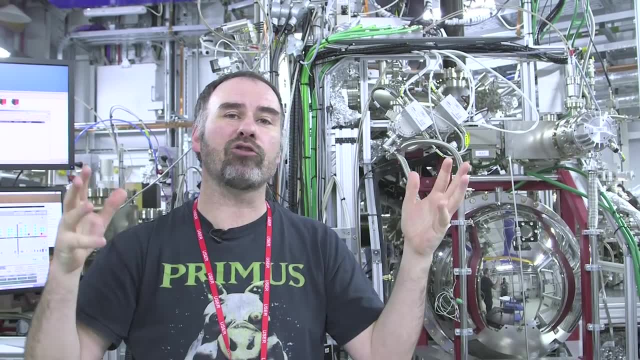 are actually going to make it through, And then we vary the voltages and we can collect a spectrum that way, So that acts like a filter. Precisely, That's exactly what it does. It's an energy filter, So it allows us to detect how many electrons we've got at a certain energy All. 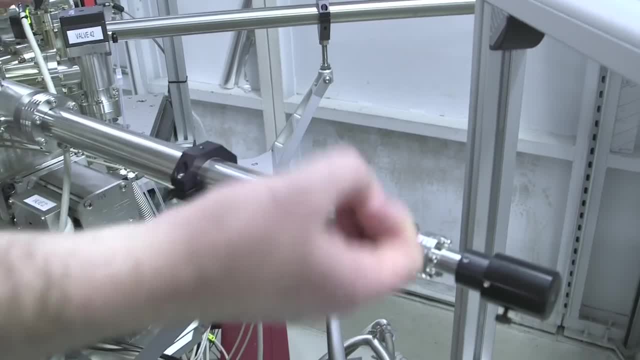 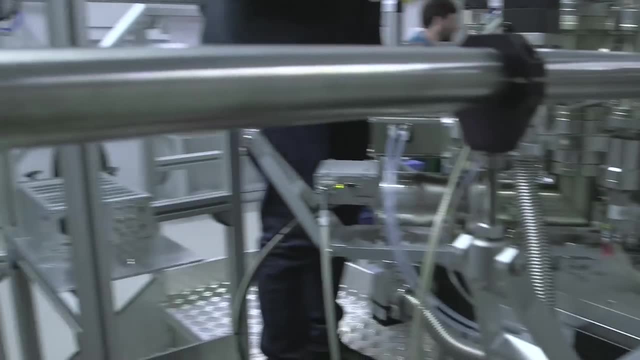 these different arms. you can see. those are allowing us to move samples around in vacuum without breaking the vacuum, And so we can use these arms to move the sample around. What they're doing over here, what Sam's doing at the moment, is sorting out the important. 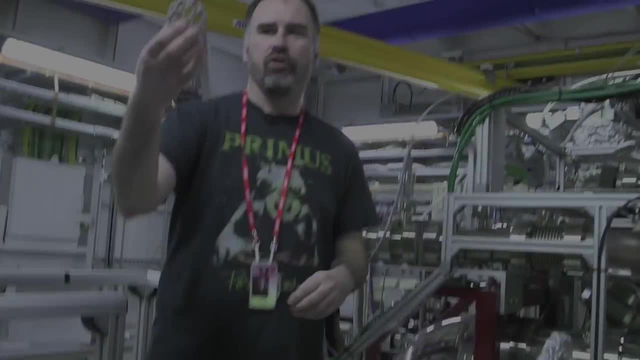 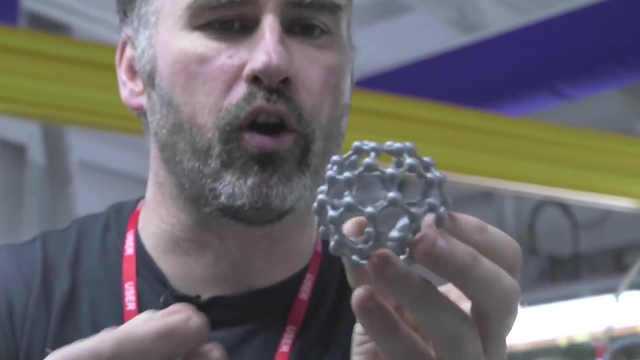 aspects of this experiment. Let me tell you about the experiment we're going to do. So this is the molecule we're interested in. It's an absolutely fascinating molecule. It's a C60.. It's what's called a buckminsterfullerene. Inside we've got a single. 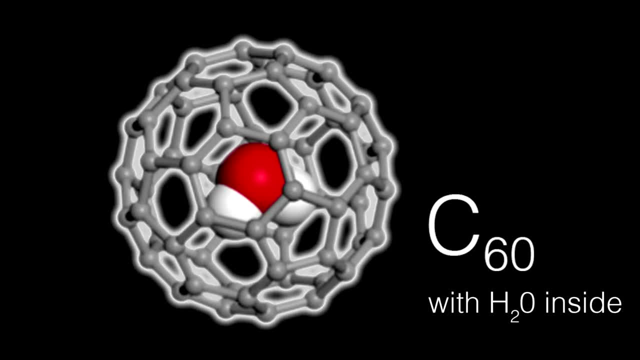 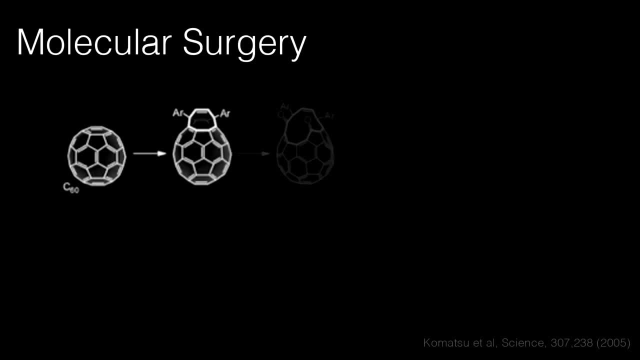 water molecule And we don't make this. We're not half clever enough. We're physicists. We're not clever enough to do this. This is made by our colleagues in Southampton. They do something called molecular surgery. They open up a hole in the cage. they drop a water molecule in. 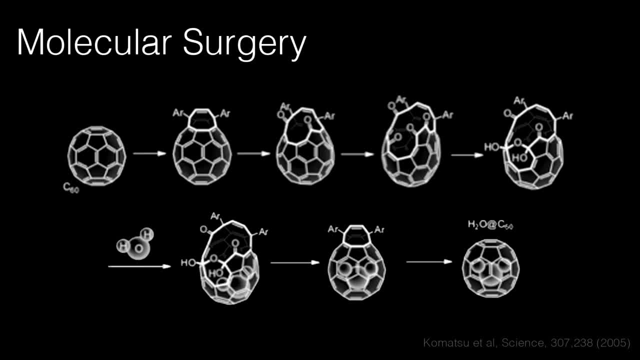 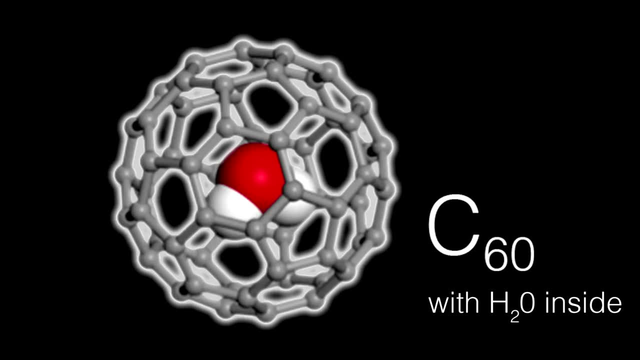 and then they seal up the hole just with wet chemistry. It's phenomenal: The water molecule is trapped within a cage, It's encaged, It's incarcerated within this molecule. Why is that interesting? Well, first of all, you've got a single water molecule. 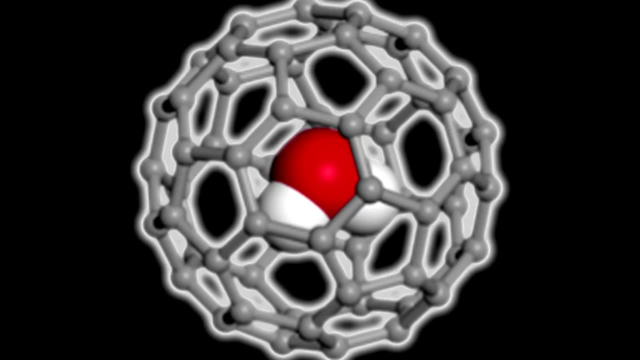 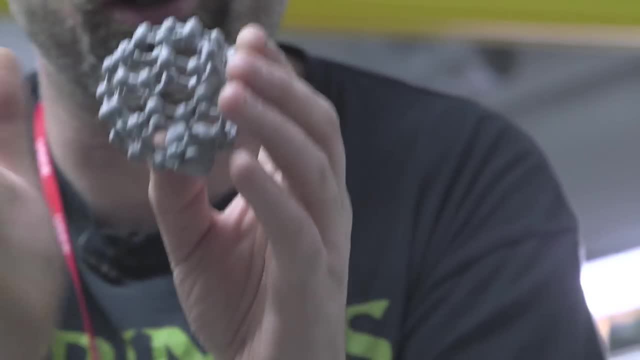 It's not interacting with any other water molecules. This is not something you find very often in nature. The C60 is about a nanometer across. Once you confine molecules, once you confine atoms, once you confine particles to small spaces, that's when you start to see very 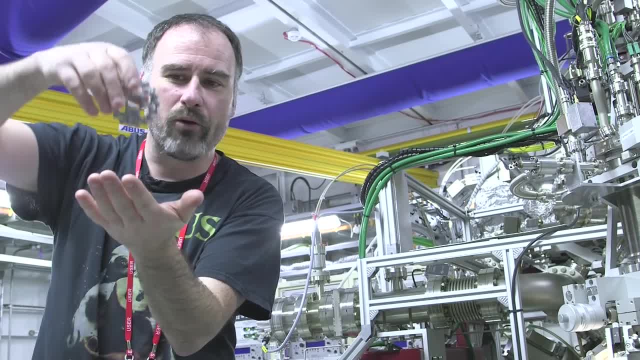 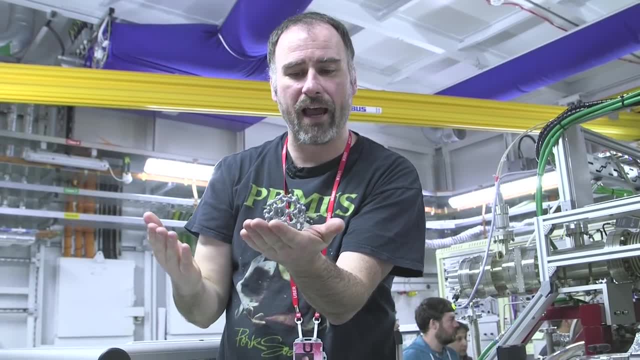 interesting quantum effects. What we're really interested in is: can we exploit those effects when we take this molecule and put it down onto a surface? And the first question to ask is: when you put it down onto a surface and the cage bonds to the surface, does the molecule 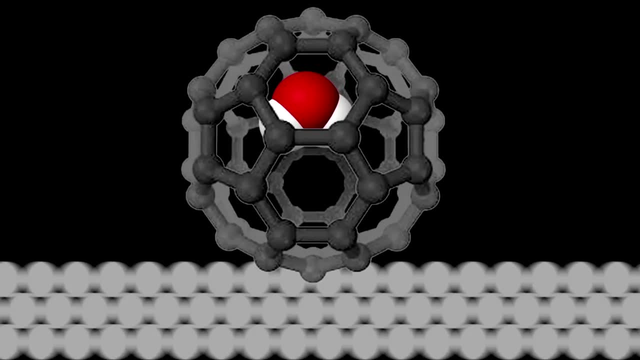 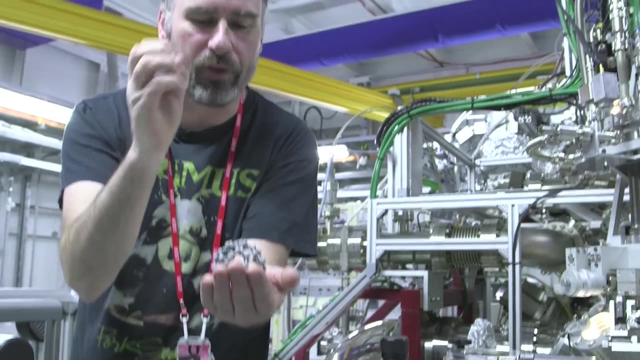 inside? does the water molecule feel the effect at the surface, Or is this just like a Faraday cage? Does it completely screen it out, so that the water molecule doesn't see the surface? There are a number of different things we do, but the first is to exploit this photoelectric effect. this 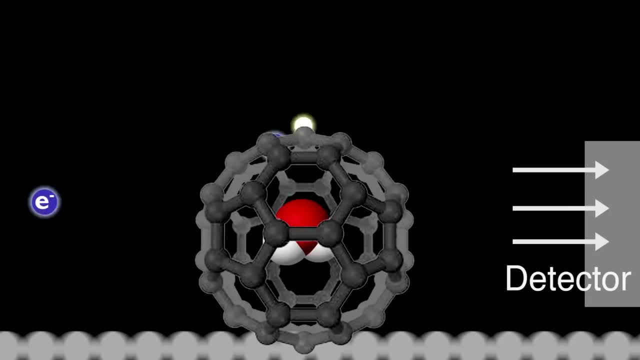 photoemission effect. Photons come in, we excite electrons out of the oxygen and we can look at the spectrum of those electrons to work out what's happening with the water molecule. Where do we get those photons? Well, we get them from the beam line. Why do we need the beam line and why is a? 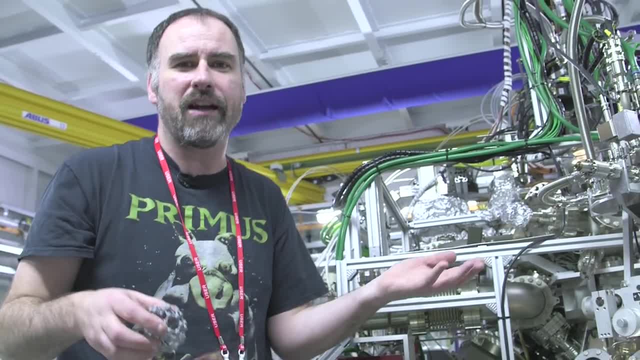 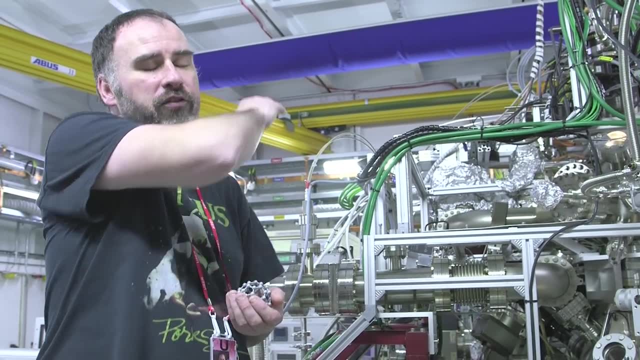 photon. why don't we just do this with an X-ray source back in Nottingham? Why don't we do it in a lab? The great thing about a synchrotron is that you can tune the photon energy across a very wide range, in this case from 100 electron volts up to kiloelectron volts. That's a remarkable tool. 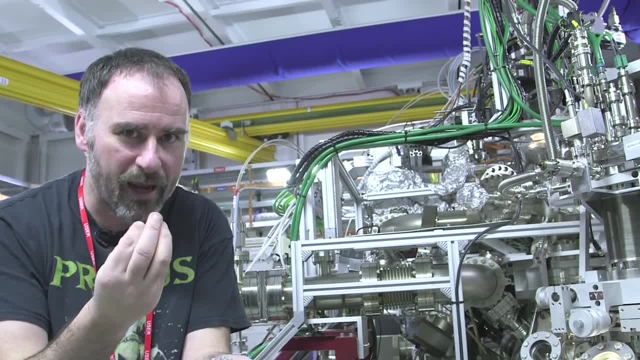 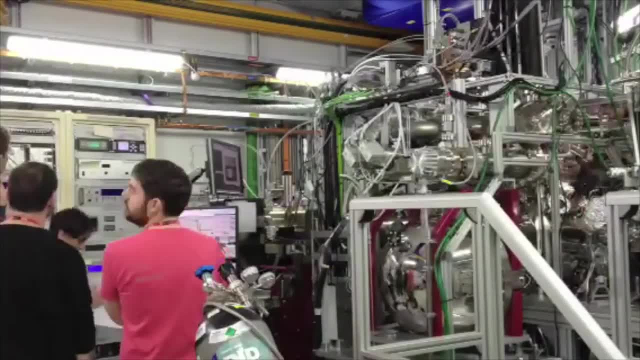 because we can tune in on particular parts of the spectrum and work out what's going on. The challenge of this experiment- it's a really fun experiment to do- is we take a silver surface, which everybody's busily preparing at the moment. 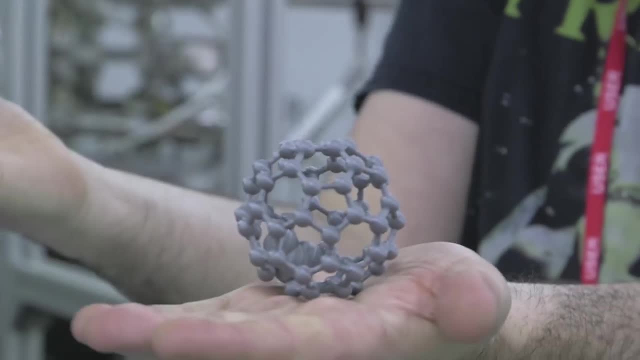 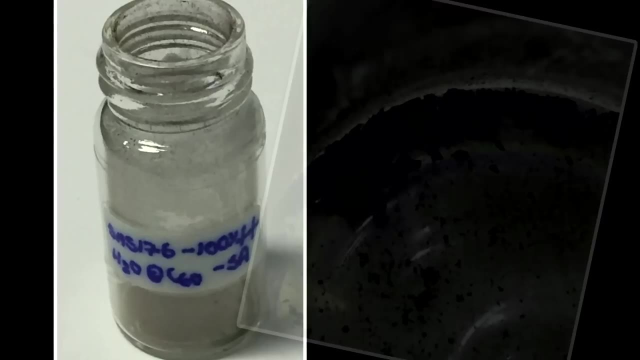 and we're going to put our molecules down onto that surface. The first challenge is: how do we get the molecules down onto the surface? Well, what we do, fortunately, with C60, we can take it as a powder and that's how we get about a milligram of these molecules. It's a black powder. 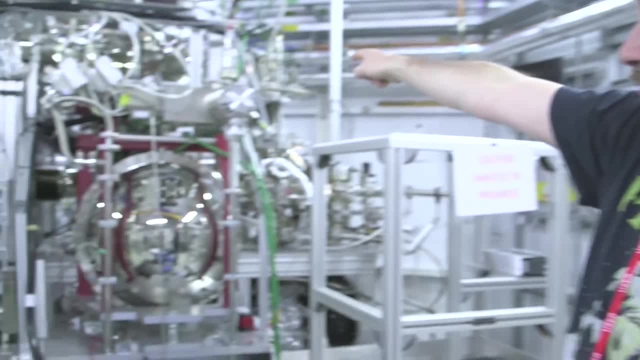 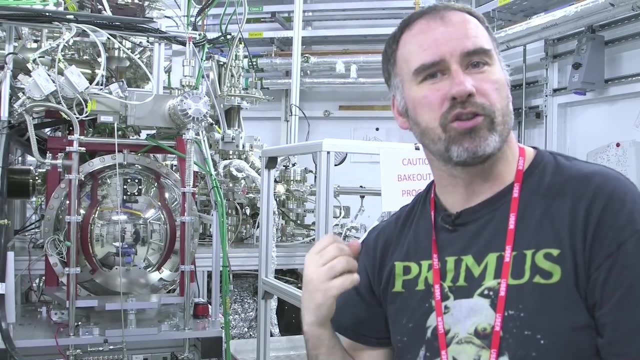 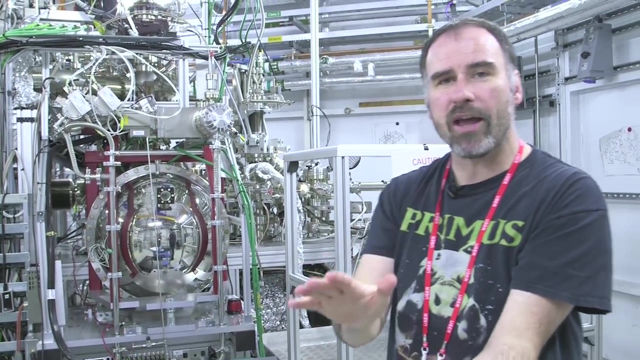 We put it into an oven- it's literally an oven- and we bolt it onto the chamber, we heat it up and the molecules very nicely sublime. They go directly from the solid phase to the gas phase and they stick. And if we do that in just the right way, it's taken us a bit of time to work out just what. 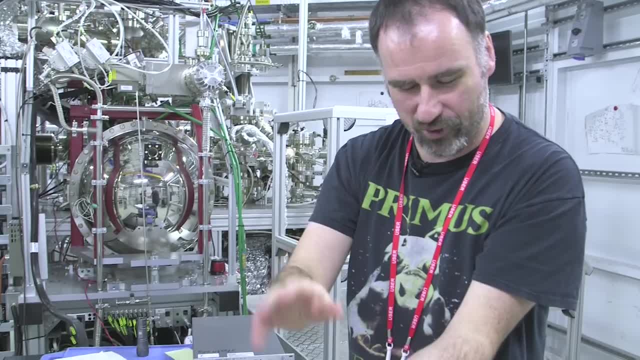 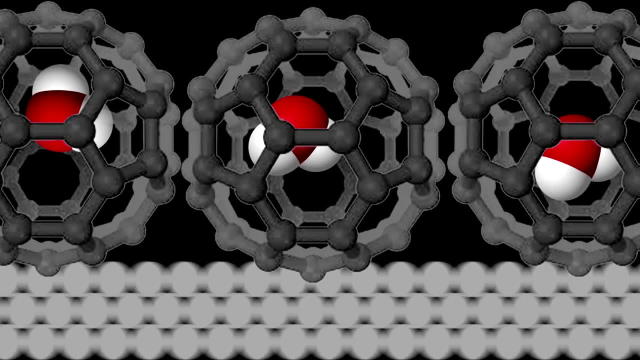 that right way is. but if we do it in just the right way, then you can get a nice ordered film, an ordered monolayer, a single layer of molecules on the surface. Then we take our beam of photons, they come in and we look at the electrons that are given out by the water. We're also interested. 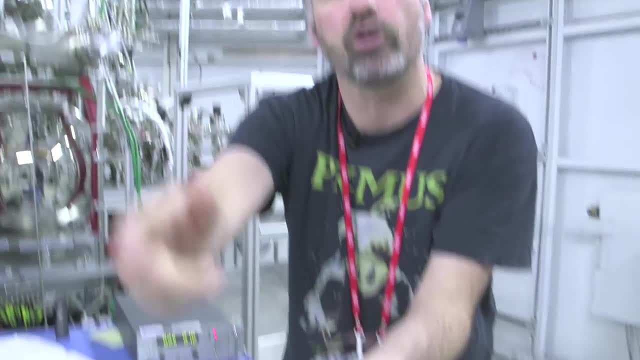 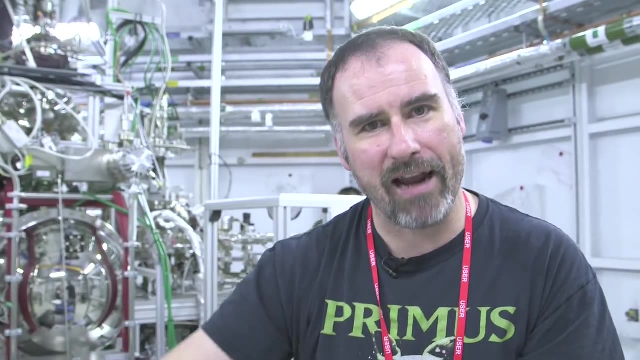 actually in the cage itself. so we also look at the electrons coming out from the carbon. That's the first stage of the experiment. But actually the technique we're going to use is we're using here in parallel and a real advantage of this particular beamline, because it can do this. 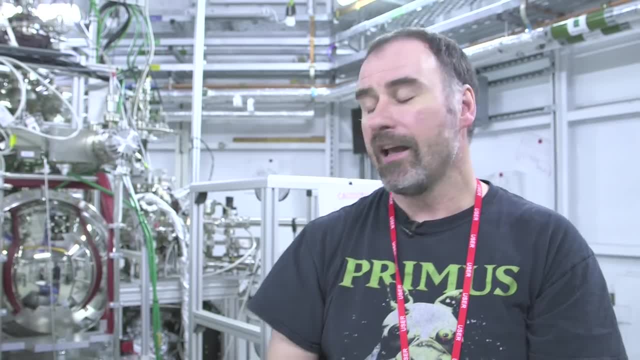 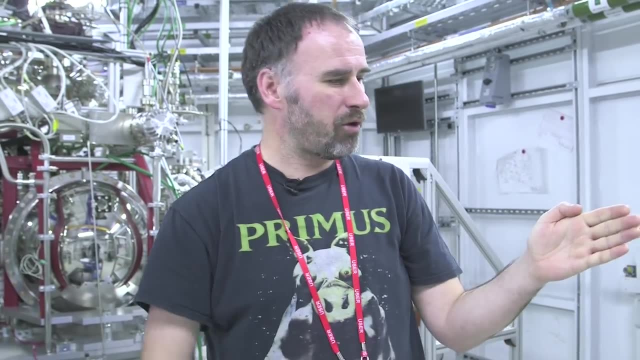 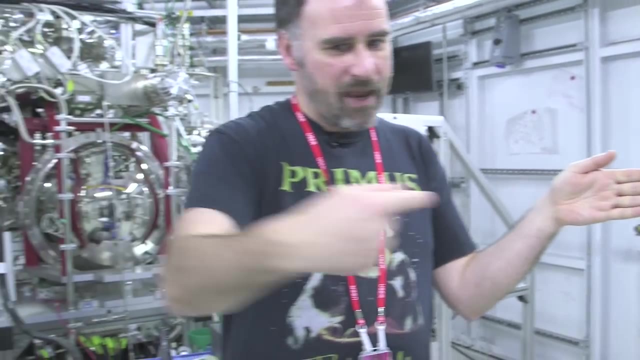 technique is something called X-ray standing wave analysis, And that's. that is a fascinating technique, And here's where my lack of a crystal comes into play. What we do is we have a crystal, there's the surface of a crystal, We have planes of atoms. What we have here is our beam coming in. 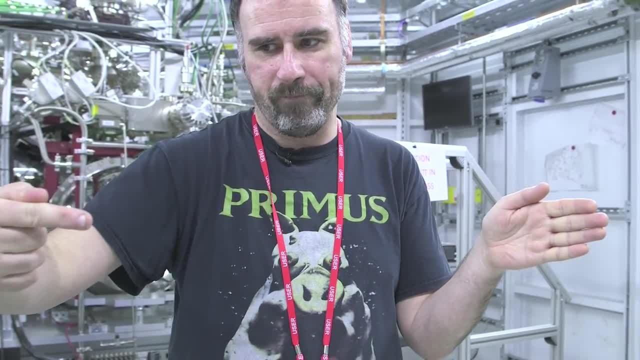 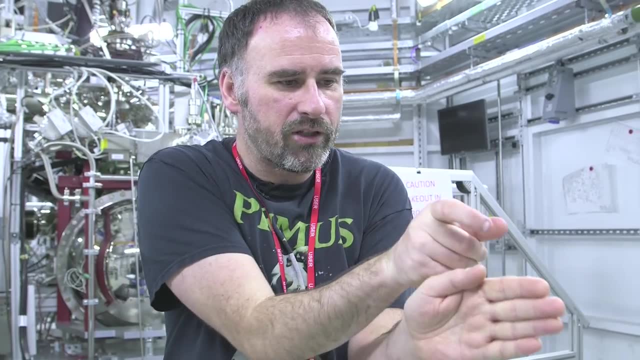 Now, if we tune our photon energy of our beam to something called the Bragg condition right, what that means is, if we get the wavelength of our beam, so it's the right, it's the same size as the spacing of the crystals. what will happen of the crystal planes? 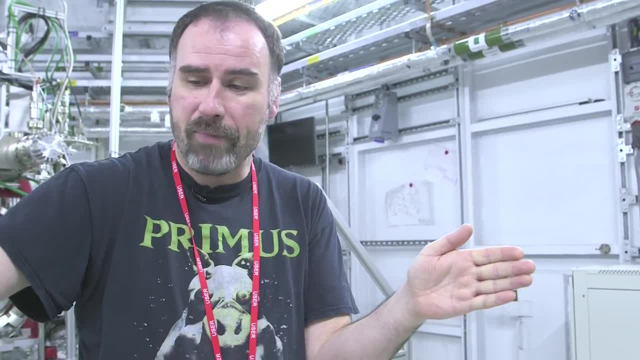 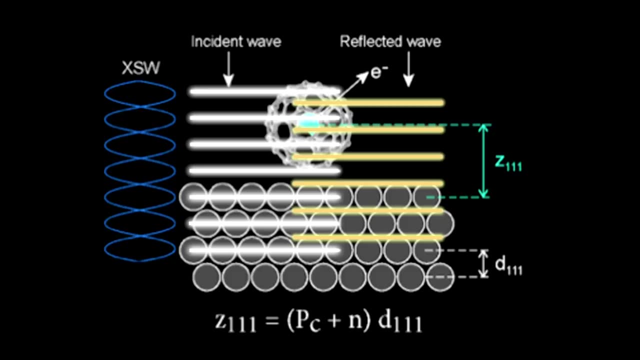 what will happen is that the beam will get diffracted. So we have a beam coming in here and we have a beam diffracted which comes back out, And when those two beams interfere, what happens is we get something which is called a standing wave. It's pretty well exactly what. 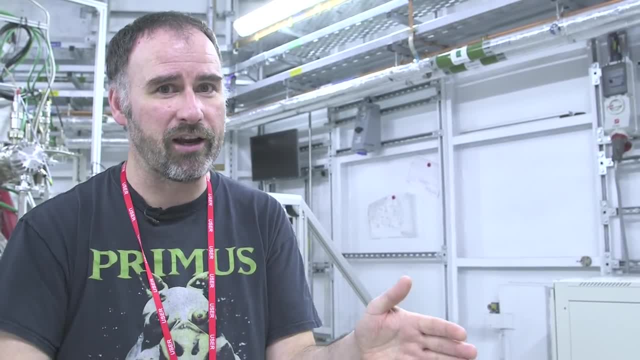 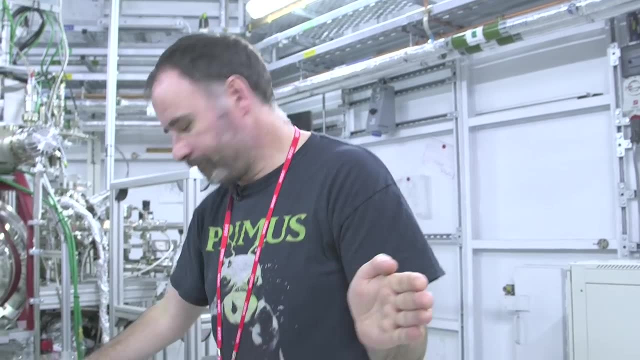 happens on a guitar string. You get a standing wave set up in a guitar string in terms of the interference of traveling waves on that guitar string. And now the great thing is, if we have our molecule at the surface, we have this standing wave field which has got a periodicity. It's a 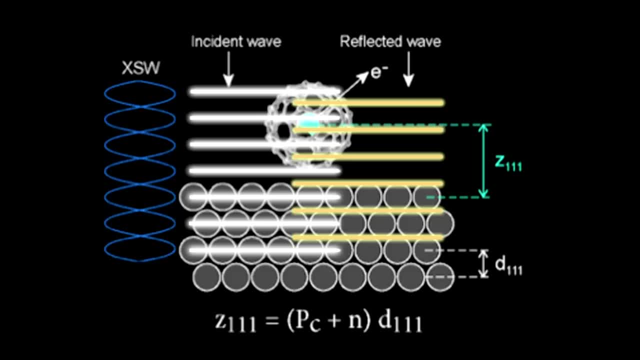 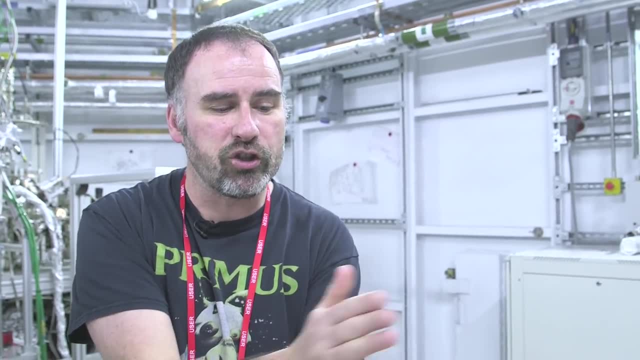 wave, so it's got a periodicity, The molecule bathed in this wave. that's the best way of thinking about it. You've got the molecule which is sitting in this wave field and if you change the energy of the incoming beam just a little bit, what you can do is you can tune the maxima and 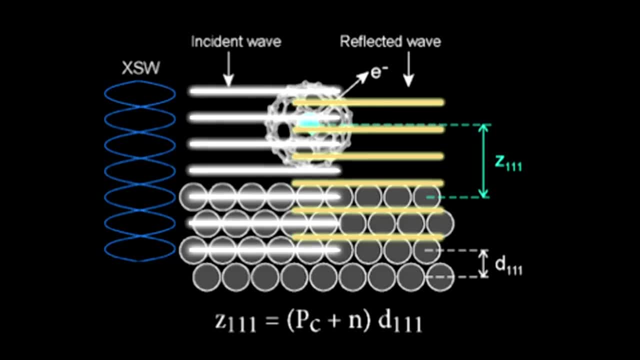 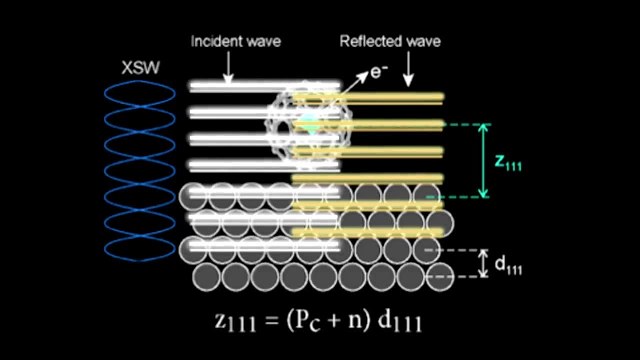 then you can move them back and forth, And by shifting them back and forth you shift them back and forth through the oxygen And then what happens is, if you look at the electrons coming out from the oxygen, you will see a characteristic profile depending on where the water molecule 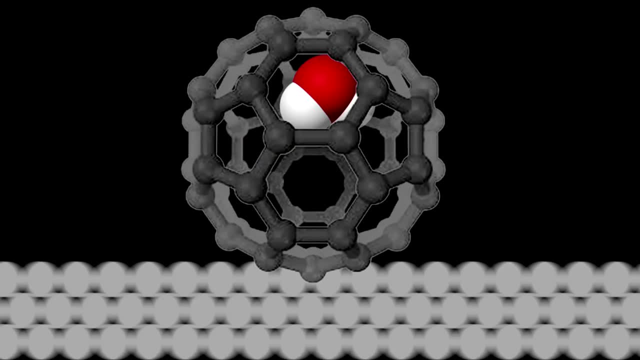 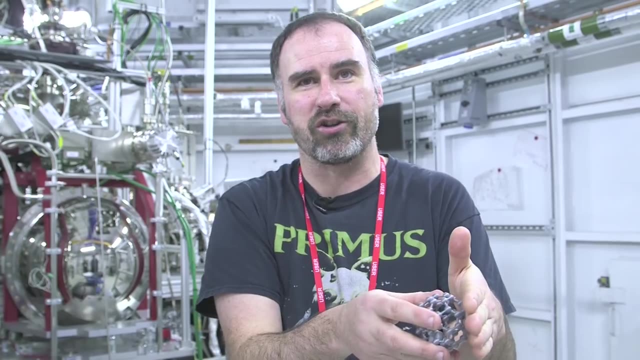 is sitting with respect to the surface planes, The reason we're doing all of this is to find out where in the cage the molecule is sitting, And, moreover, we're not even restricted to those planes. What we can do is we can rotate our sample and we can triangulate the position. 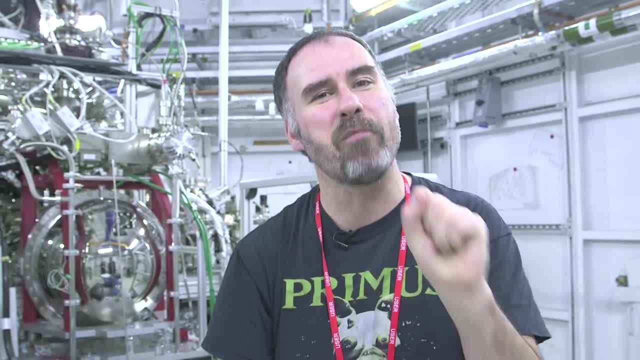 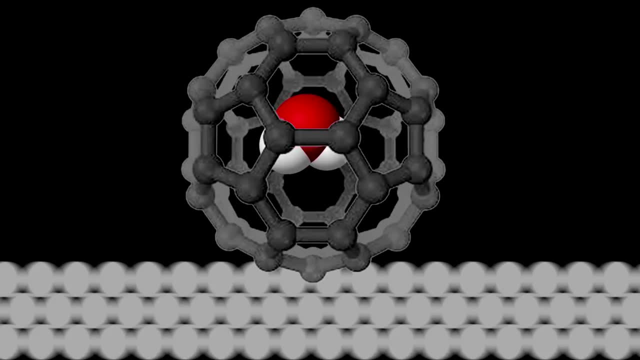 of the molecule. We can do the same thing again and triangulate the position of a single molecule within the cage. We have done some preliminary work. We're fairly confident it's going to be sitting fairly close to the center of the cage, which is relatively surprising because when these 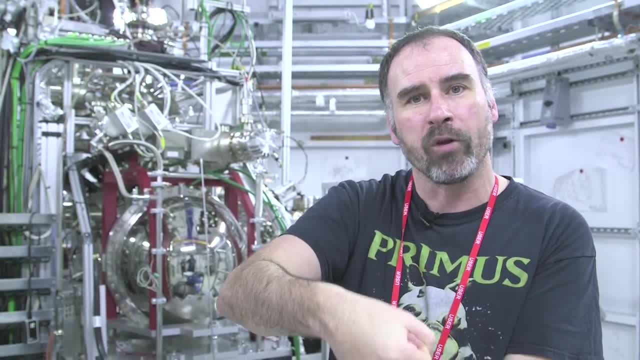 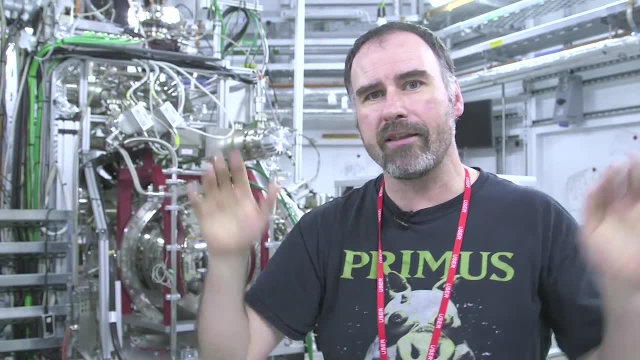 molecules. when the fullerene molecules go down onto the surface, what happens is those charge from the silver surface. electrons go into the molecule, forms a quite strong bond, and yet the water just sits in the middle of the cage, going I don't care, which seemingly does, It seems to be. 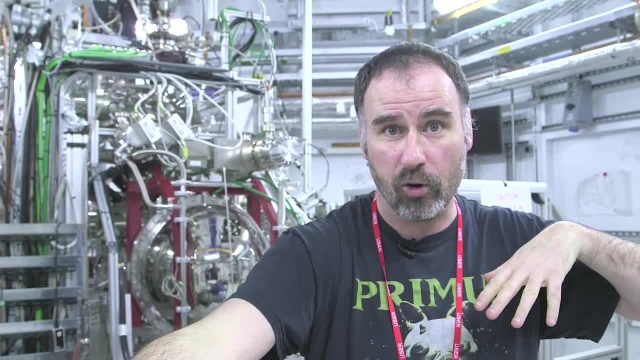 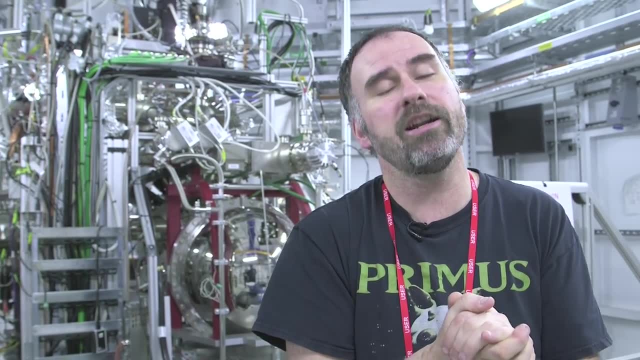 interesting to see that the water just is not going to touch the screen from its environment, which, in terms of actually being able to exploit this effect, to be able to look at that water molecule and exploit in the device, for example, is really quite interesting. We're locked in. 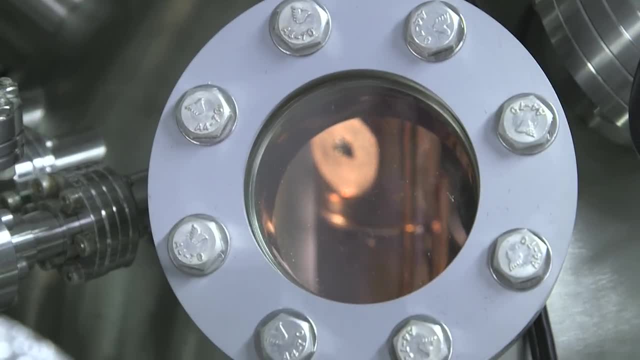 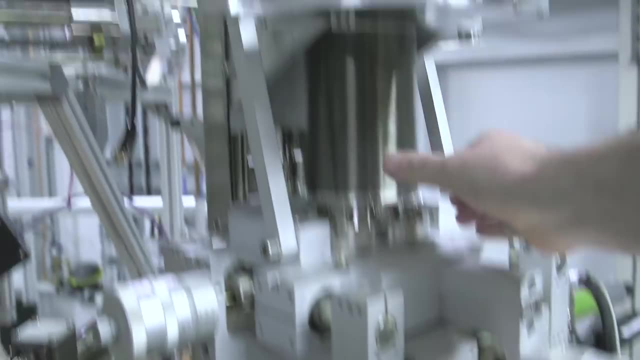 So they're going to turn the beam on. We'll be fried. we'll be absolutely fried. You're looking into the chamber, absolutely So. you're looking into the preparation, one of the preparation chambers. This thing coming down with the bellows is a manipulator that allows us to move.